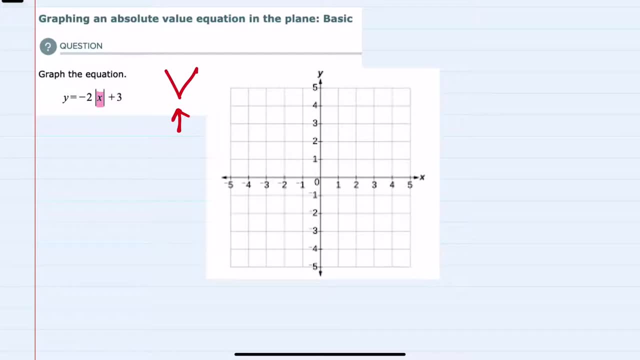 we know that the point of the v will happen at x equals 0. And so, to graph this, I'm going to plug in a 0 for x, but I'm also going to choose a couple of points to the left of that. Minus 1 and 2 will work. 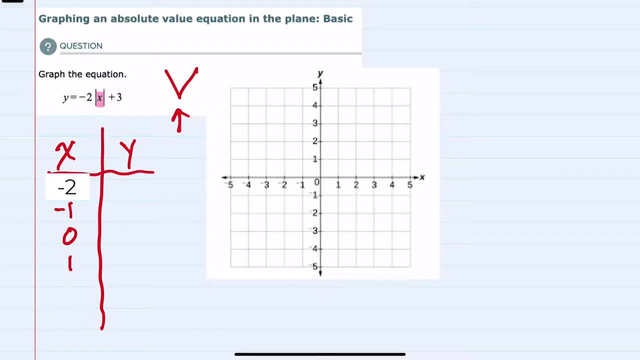 And a couple of points to the right. So I'll use a positive 1 and a positive 2. And plugging those values in, I'll start with: x equals 0. When we plug that value in, we will have y equals negative 2 times the absolute value of 0 plus 3.. And then, following the order, 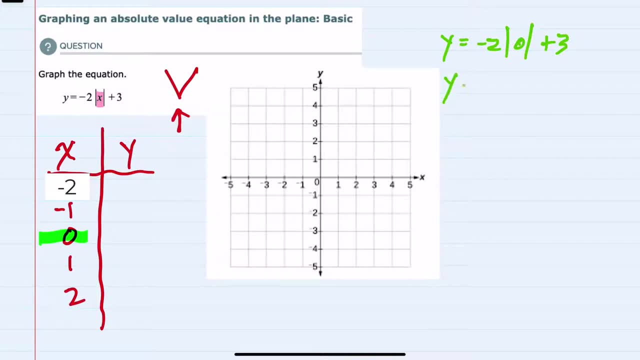 of operations. the absolute value is a grouping symbol. so the absolute value of 0 is 0.. Next we move on to multiplication. Multiplication negative 2 times 0 is also 0. So we have y equals 3 when x is 0. So so. 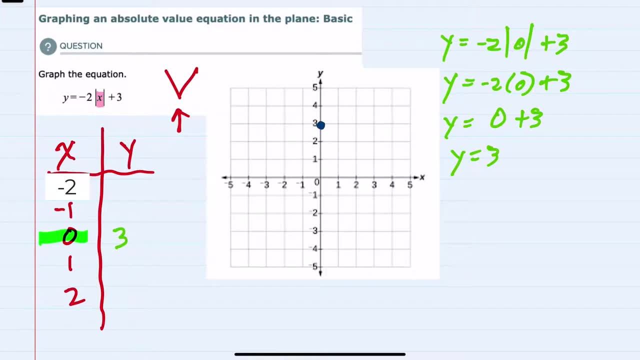 far we have the point 0, 3.. Next I'll try 1.. So when we let x equal 1 and we substitute into the equation, y equals negative 2 times the absolute value of 1 plus 3.. Again, the 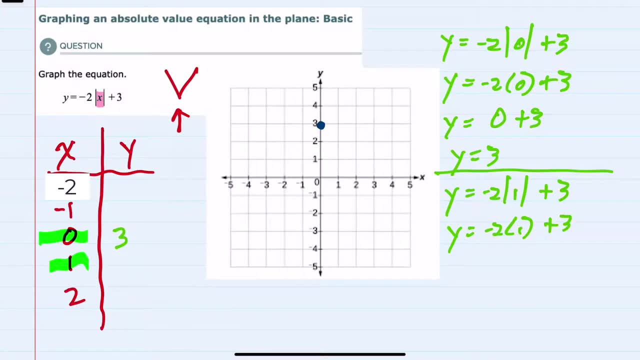 absolute value of 1 is 1.. Moving to multiplication, negative 2 times 1 is negative 2.. And then negative 2 plus 3 is 1.. So we have the point 1, 1, which is here. I'll continue with the positives by doing 2. next, When I substitute 2 in for x. 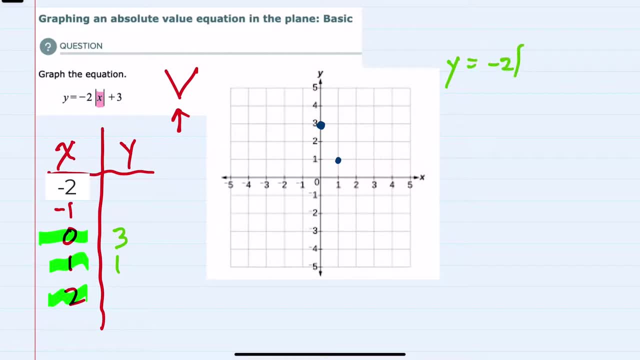 we get: y equals negative 2, absolute value of x, which is now 2, plus 3.. The absolute value of 2 is 2.. And then, multiplying negative 2 times 2 is a negative 4.. And when we add: 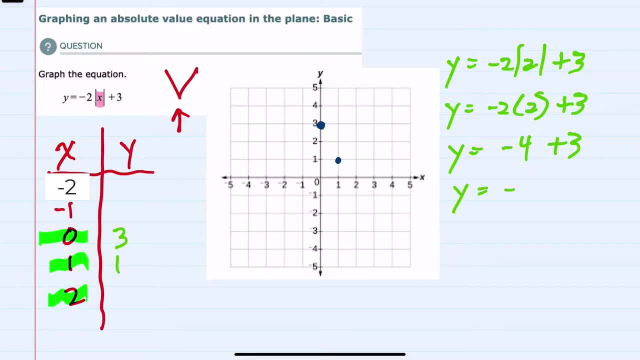 the 3, we have y equals negative 1.. So our next coordinate is 2 negative 1, which is here, and we'll next move to substituting in these negative values of x, starting with negative 1.. Substituting for x, we would have y equals negative 2 times the absolute value of negative 1 plus 3. and here when